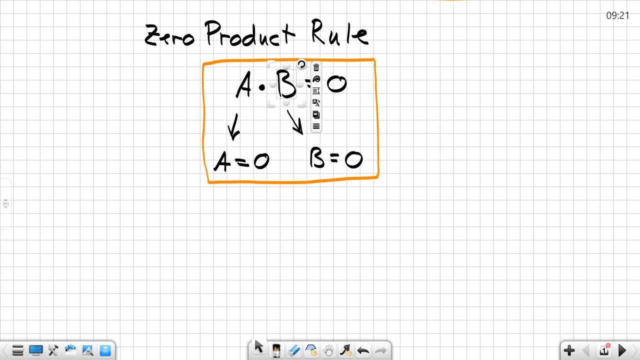 I have two factors, some a multiplied by some b, and the result is zero, then it has to be so that either the first one is equal to zero or the second one is equal to zero. If you are thinking about numbers, then this becomes very clear. For instance, 3 times a number that I am thinking of, and 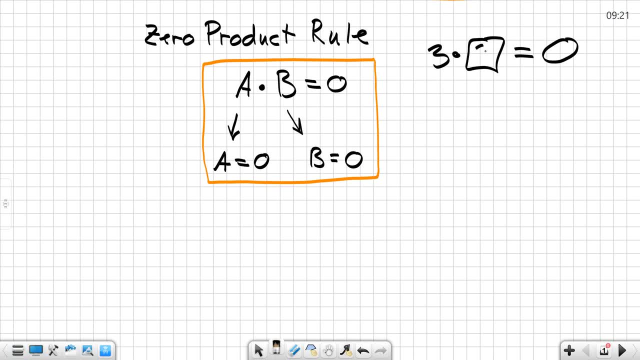 the result is equal to zero. Well, what number can this possibly be? Well, it has to be zero because otherwise you won't end up with zero on the right side. And this works in the same way if the first number is some mystery number and I multiply it by, let's say, 5 and the result again is zero. This number in here. if I multiply it by 5, then it is equal to zero. This number in here. if I multiply it by, let's say, 5, and the result again is zero. This number in here. if I multiply it by, let's say, 5, and the result again is zero. This number in. 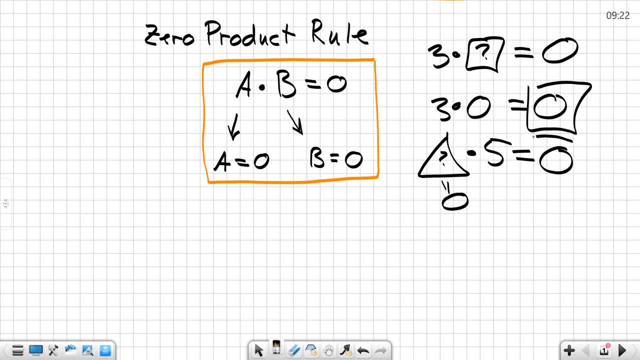 here, if I multiply it by, let's say, 5, and the result again is zero. This number in here it has to be equal to zero, otherwise the product altogether cannot be zero. So let's go ahead and use this. let's solve our first equation. Now, the first equation is going to be fairly. 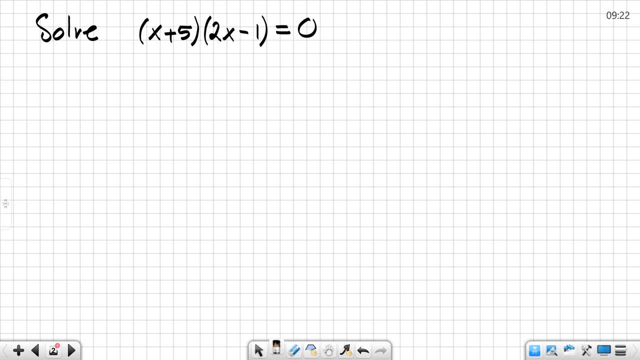 simple, because it is already in its what we call the factored form. I have x plus 5, multiplied by 2x minus 1, and the product is supposed to be equal to zero. So let's draw the sum. What are we going to do? 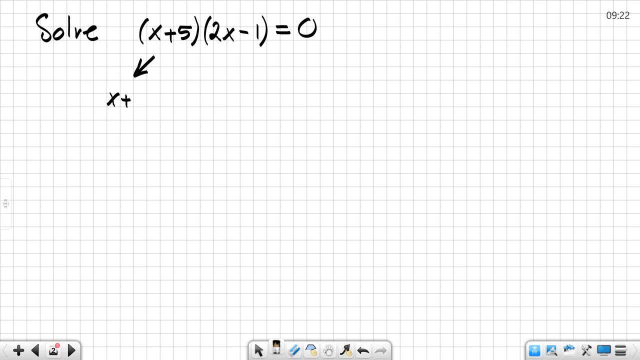 Well, I'm going to take my first factor, x plus 5, and I set this one equal to 0.. And I take my second factor, the 2x minus 1, and I set this as well, equal to 0. 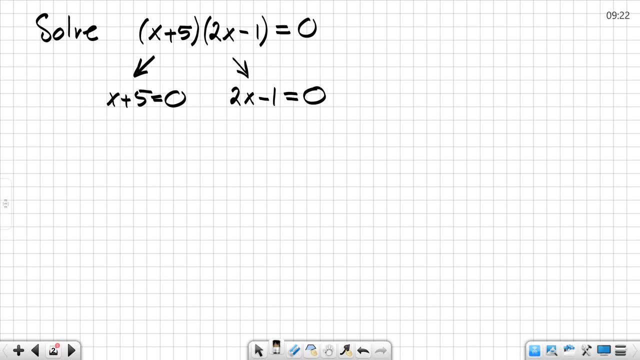 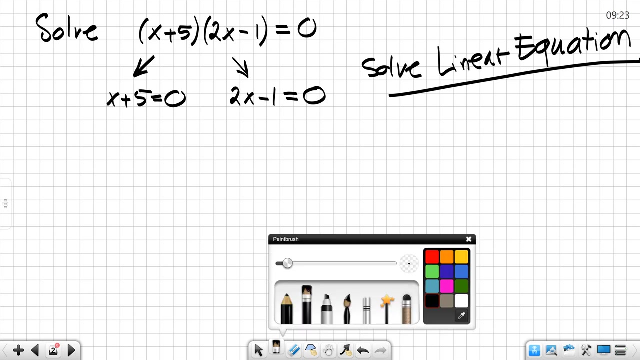 And now what we are just going to do? we are going to solve these, what we call linear equations, And that is always going to be something fairly simple. We know how to do this, So here's the trick: Instead of solving a quadratic equation, I will split it up into two factors and solve two linear equations as well. 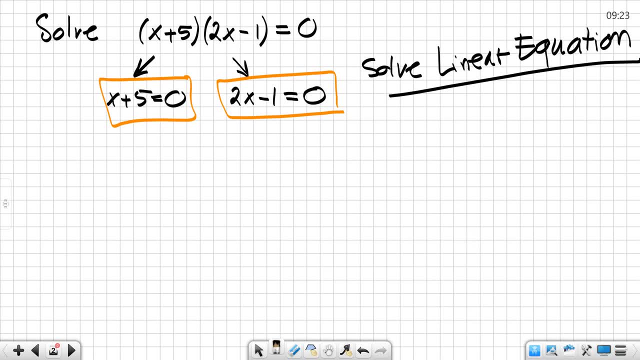 So this is going to go fairly quick. In the first case I just subtract 5 from both sides And I get that x has to be negative 5.. In my second equation I first take the negative 1, I move it to the right side by adding 1.. 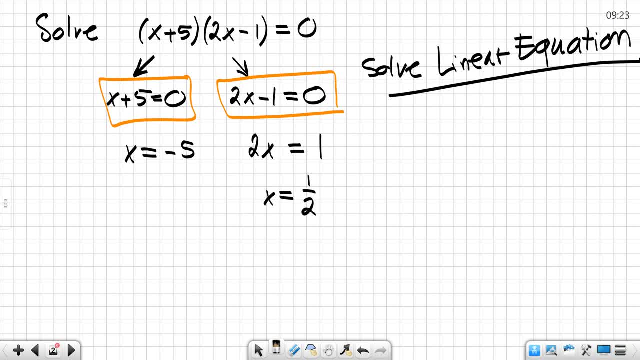 And now I'm dividing both sides by 2, and I get that x is equal to 1 half. So, and you see already now that I'm not writing those in-between steps down anymore, We are getting, we are speeding up a little bit. 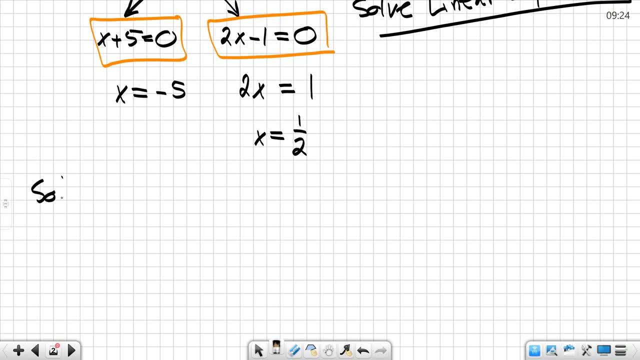 So what does this mean now? It means that the solution set looks like this: I have two numbers in my solution set, The numbers negative 5 and 1 half. Let's do another one. We want to solve: x squared plus 3x is equal to 4.. 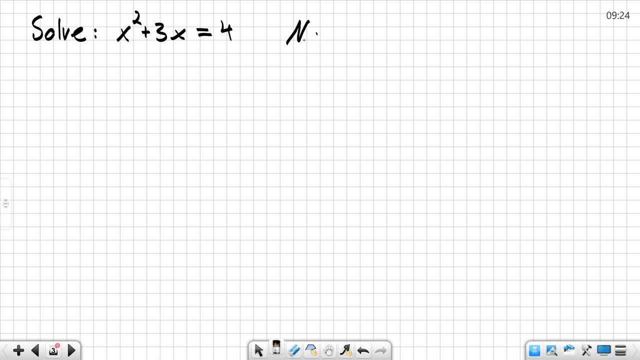 This is linear equation. It's not in standard form yet, So what do I have to do? I need to bring it in standard form, And that means it has to be equal to 0. This can be easily done. Let me write it down just one more time. 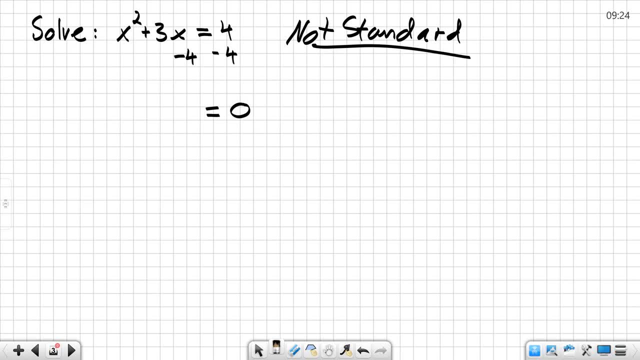 Negative 5.. I'm subtracting 5 from both sides. You really do not need to write this step down if you can just take the positive 5 and move it to the left by subtracting 4.. Alright, Now I have it in standard form. 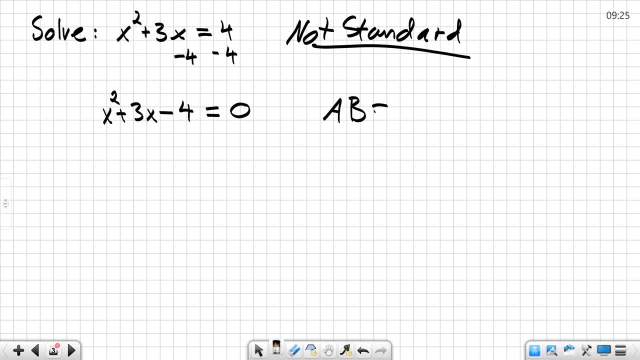 And now I need to have it in this way that I have something times, something else is equal to 0. So I am factoring. Let's have a look: Two numbers that multiply together give you negative 4. But when you add them gives you positive 3.. 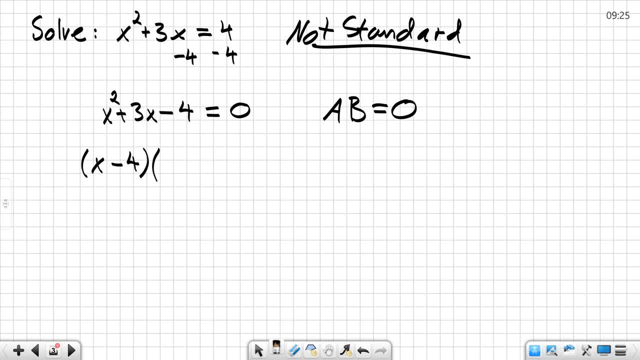 Would be a negative, 4. Positive, 4. And a negative. 1. Checking 4 times: negative, 1 is negative, 4.. 4 plus negative 1 will be positive. 3. Works out So now what I'm going to do. 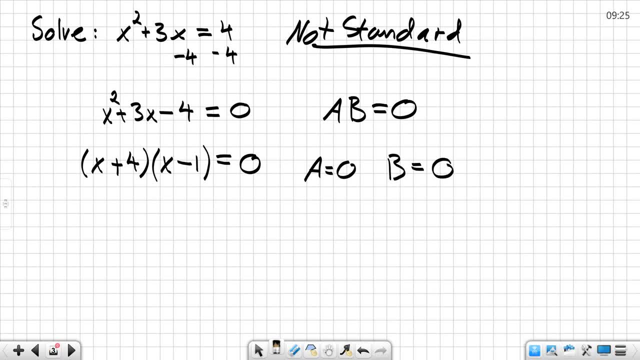 I just simply set both factors equal to 0 and solve those linear equations. So either x plus 4 is equal to 0.. Or x minus 1 is equal to 0. And you see that these ones are really very simple to solve. 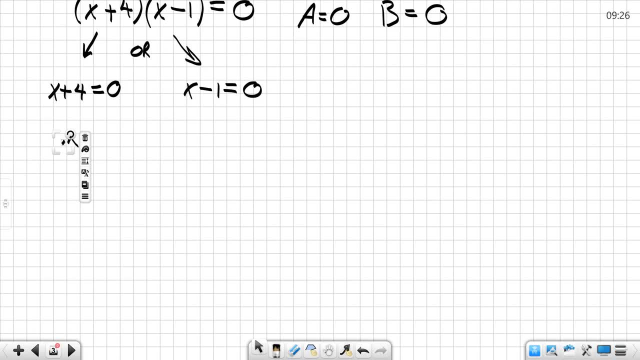 I subtract 4.. Whoops, Let's eliminate that. I subtract 4 on the left equation and on the right equation I'm adding 1.. And that means now I have found two solutions, And my solution set The numbers. 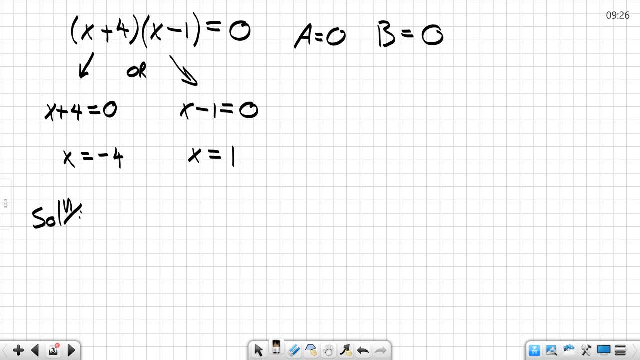 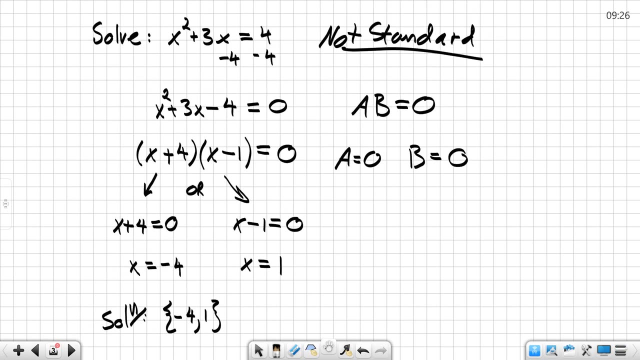 That are working. That would consist out of Two numbers, The numbers negative 4. And positive 1.. Now, What does this all mean? Why are we even bothering solving quadratic equations? Well, Let's have a look at the graph of something. 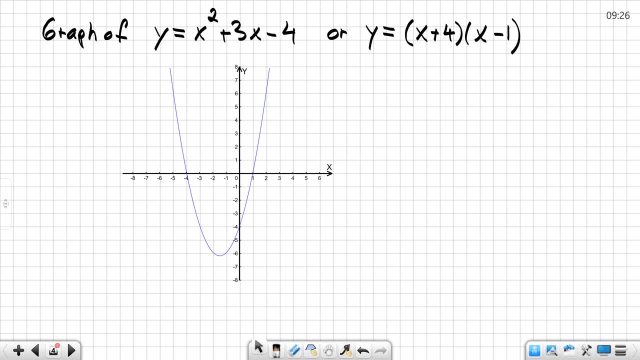 Here's the graph of y is equal to x squared plus 3x Minus 4.. Remember that we have solved this equation. Let me move this a little bit further down. We have just solved: 0 is equal to x squared plus 3x minus 4.. 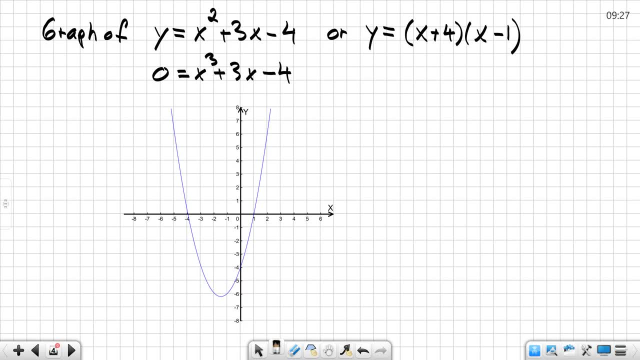 We have solved this equation. Now The graph of y is equal to x squared plus 3x minus 4.. Looks like this blue line- Or if I would draw over it right now, I will make it orange- And we notice something. 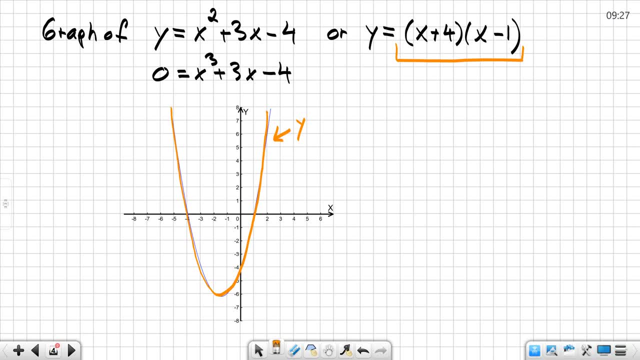 Another form of the same equation would be the factored form. This is what we used To solve this equation, And when I'm looking at the graph, I notice something. This graph, The graph of y, Crosses the x axis. 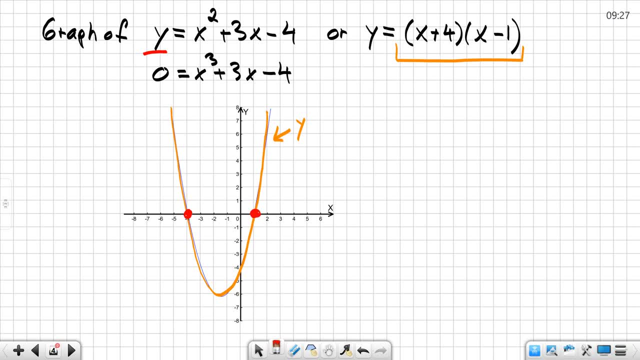 Right here And right there. And where is that? That is, at negative 4. And at positive 1. And we have just said that the solution set To this equation right here Consists out of: Well, That's an ugly parenthesis. 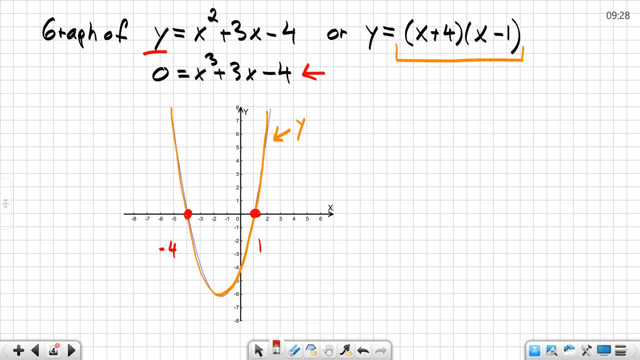 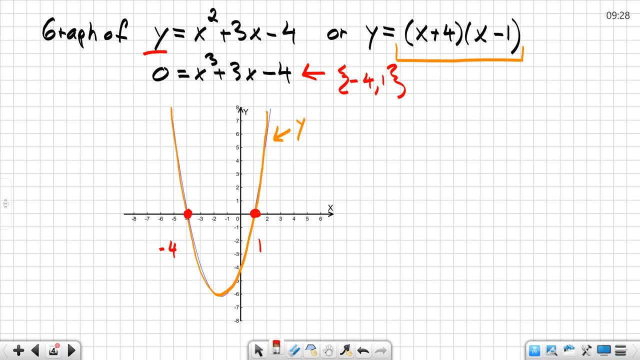 Are. The coordinates Of these points Are Negative. 4 comma 0.. This is where y Was Equal To 0.. And Right here Is the second point Where y Was also Equal To 0.. 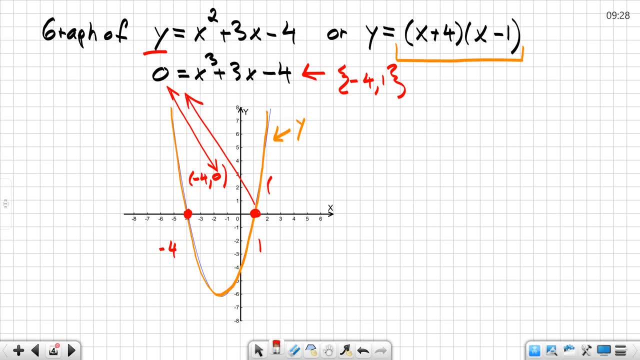 And the coordinate Of this point Is 1. Comma 0.. So The idea Is this: Solving Quadratic Equations Will Enable Us To find The Ax In The 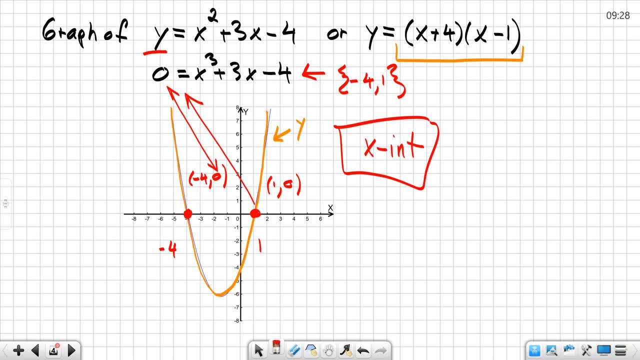 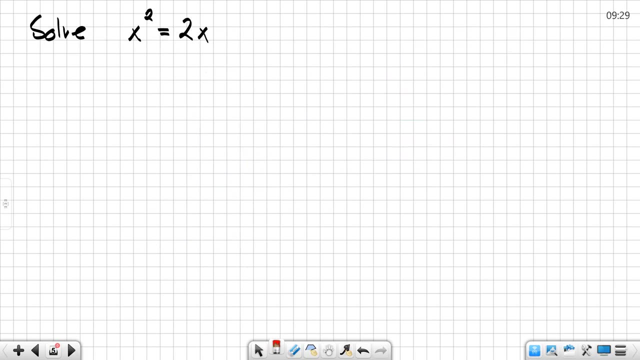 Intercepts Of The Corresponding Graphs Of The Quadratic Equation. Y Is Equal To. This Will Help Us Tremendously Later On In The Next. 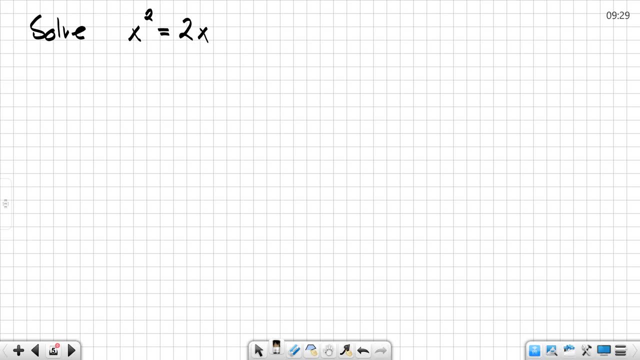 Class In College Algebra. All Right To Bring It In Standard Form By Subtracting To X From Both Sides. Now I Will Have To Factor. 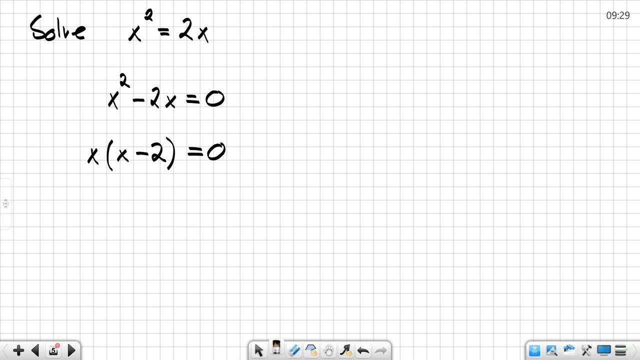 And I See That There Is A Greatest Common Factor Of Factors. Here Is The Product Of Two Things. I Do Not Need To Put A. 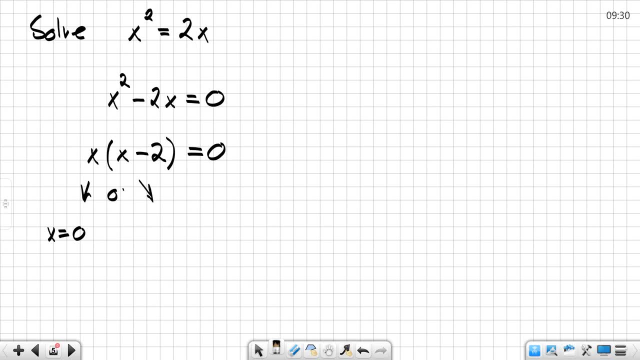 Dot In Between There. That Means That This Is A True Statement. This Is To Both Sides, So I Get That There Is A Solution. 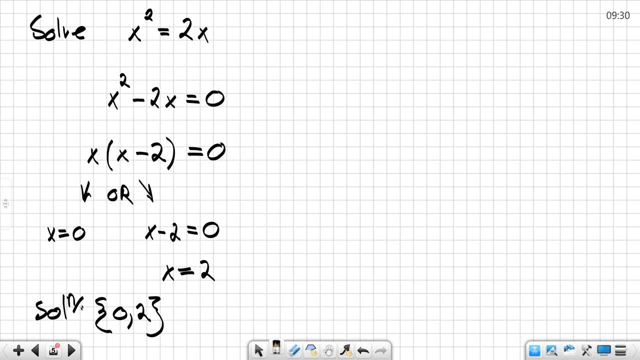 And The Solution Set Consists Out Of The Two Numbers, The Numbers Zero And Two. All Right, Let's Look At This Equation: Zero Is Equal. 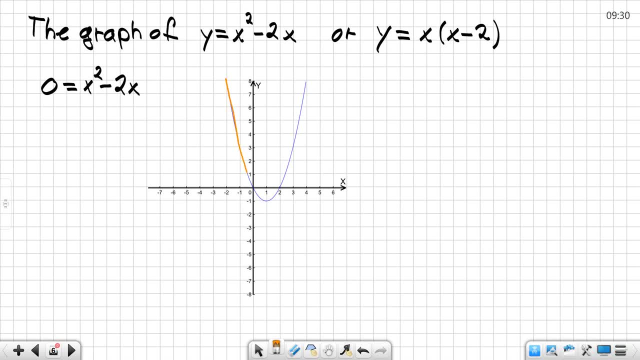 To X Squared Minus Two X. And What Do I Notice When I'm Looking At The Graph, The Picture? So To Speak Of X, 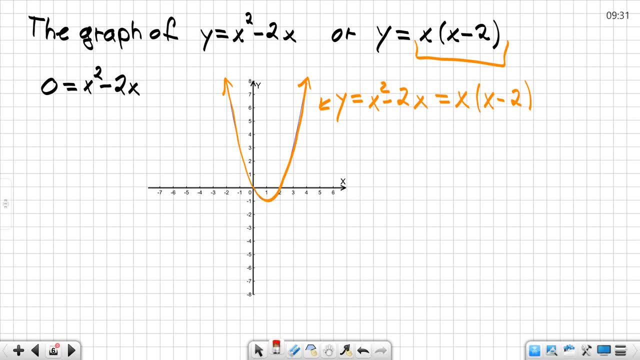 And I Notice That The Exact Same Thing Happens As Before Down Here, Where This Graph Crosses The X Axis. Those Were The Solutions To 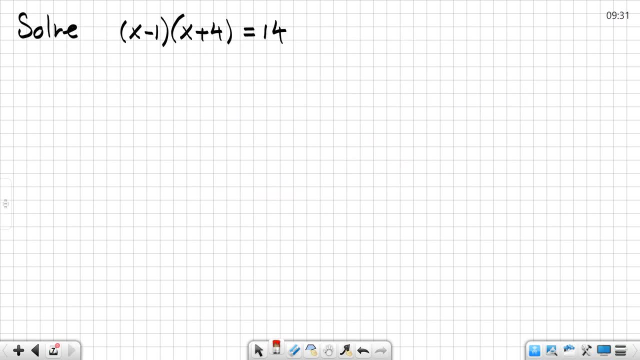 This Equation Right Here And Solve A Little Bit Of A Trickier One. So We Are Here To Solve Now This Equation X Minus One. 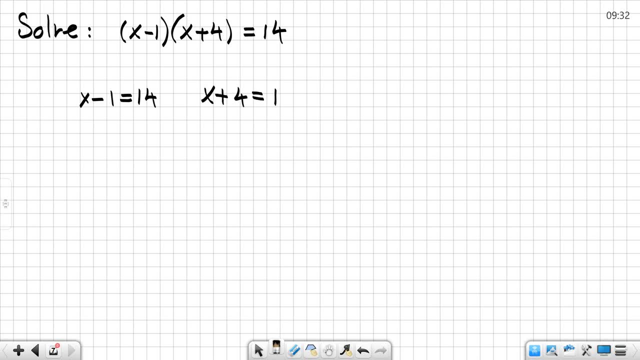 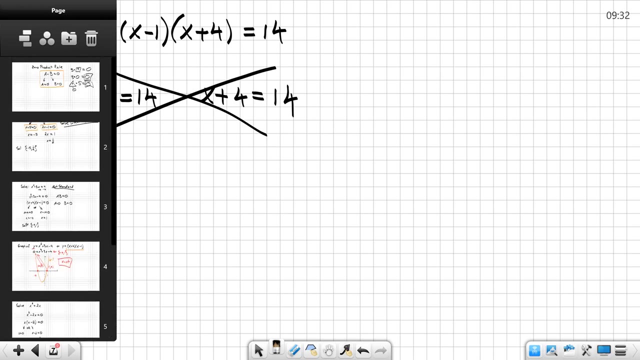 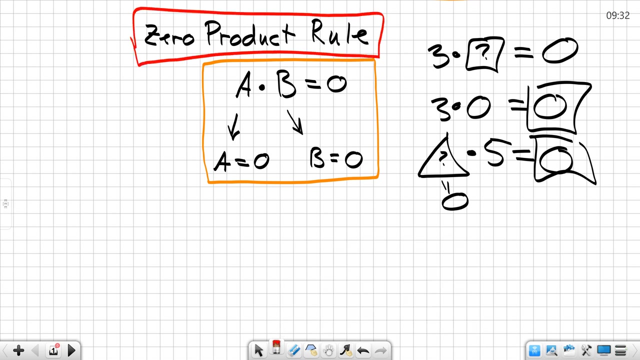 Times X Plus Four Is Equal To Fourteen. This Is Not Okay. This I Cannot Do, Because We Said At The Beginning The Principle That 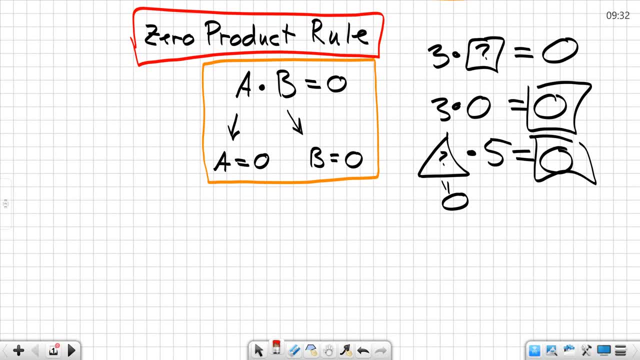 We Have Here Was Called The Zero Product Rule, Not The Fourteen, Anything. The Simplest One Would Be One And Fourteen Or Two, And 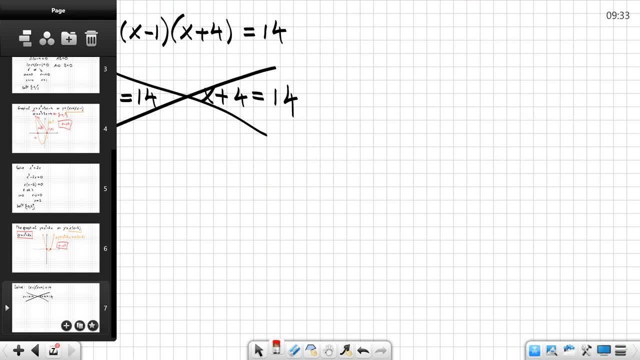 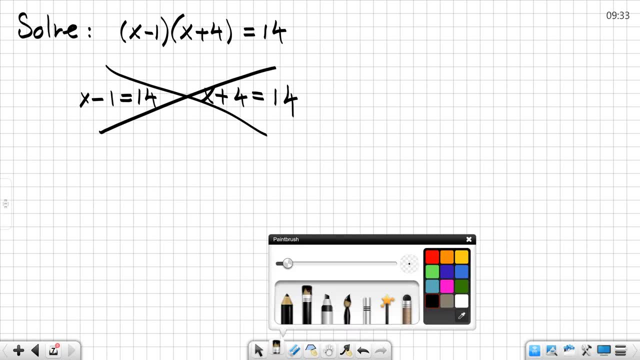 Seven, But Of Course There Are Also Many Fractions Whose Product Is Fourteen, So I Have To. The Standard Form Is The Most Important. 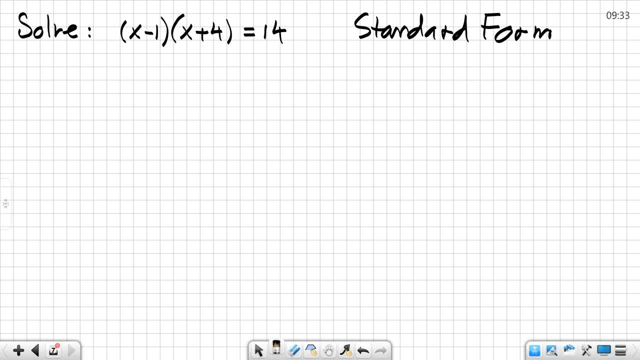 Part. So We Are Not Going To Do This Now. There Are Two Different Ways How I Can Do This. I First Outer In A Last. 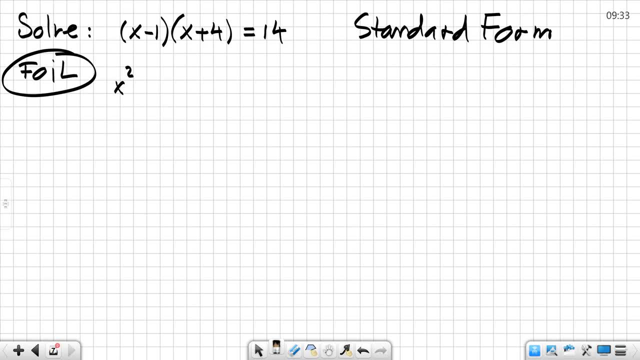 X Times X Is X Squared X Times Four Is Four X Negative One Times X Is A Negative One X Negative One Times Four. 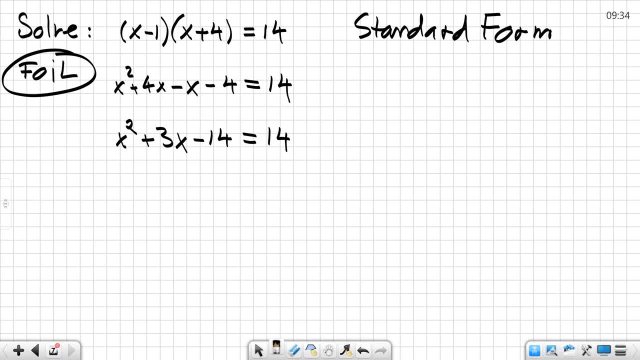 Now I'm Going To Subtract Fourteen. Maybe I Should Write This Down. Maybe I Should, Because This Fourteen On The Left Side Does Not. 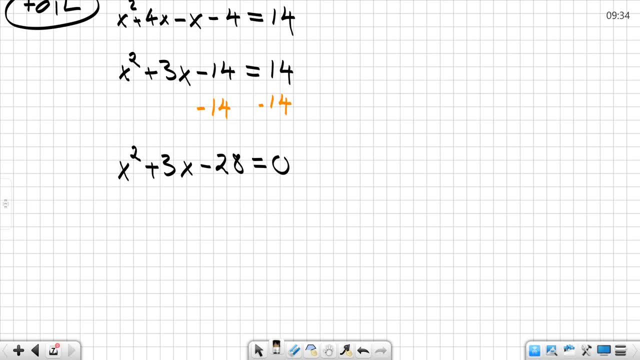 Disappear: Negative Fourteen Minus Fourteen. So I Are Going To Find Two Numbers. Whose Product Is Negative Twenty-eight? Whose Sum On The? 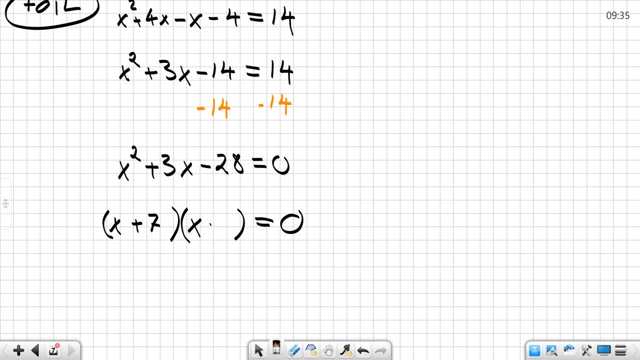 Other Hand Is Positive Three. So Can We Do This? Can We times negative 4 is negative 28,. 7x minus 4x is 3x, and x times x is x squared This: 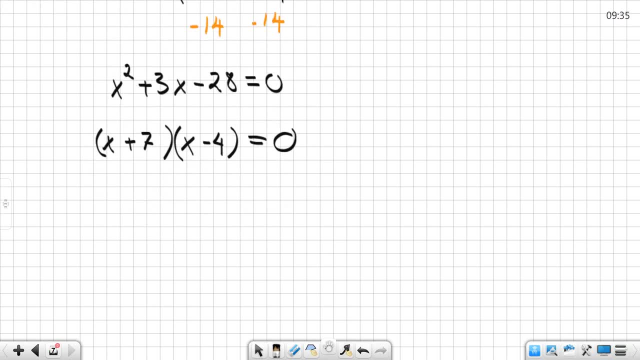 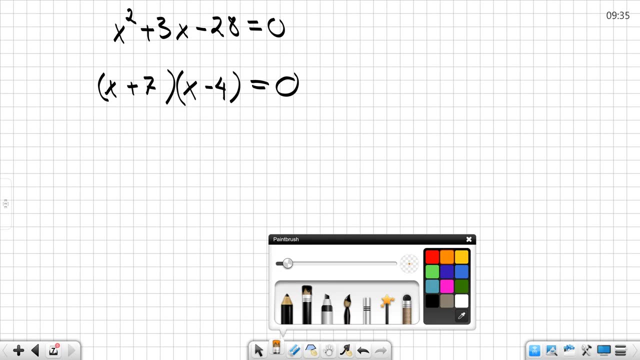 works. So the rest is a piece of cake. but we should still write down these steps, because now I have the product of two things who is equal to 0, and that means all I have to do is set both of these factors equal to 0, and then solve the corresponding linear equations.